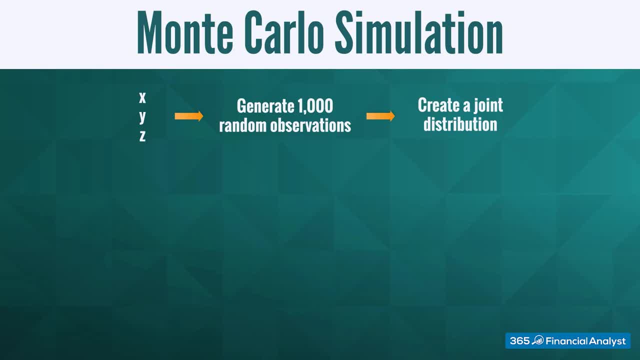 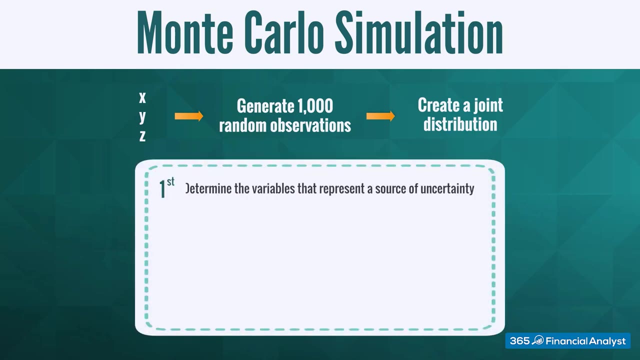 and hence create a joint distribution regarding the different possible outcomes resulting from the combination of the random variables. In layman terms, a Monte Carlo Simulation consists of the following series of steps: First, determine the variables that represent a source of uncertainty. Second, assume a distribution for each variable. 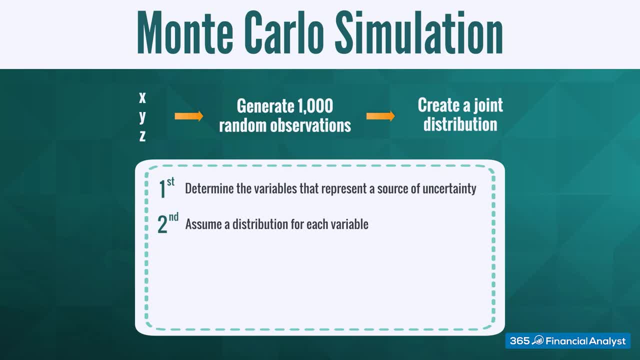 Please note that the distribution that will be chosen is up to the analyst's discretion And, of course, the final model predictions will be as good as the analyst's. The analyst's choice of distribution for the unknown variables Very good. The third step refers to the following: 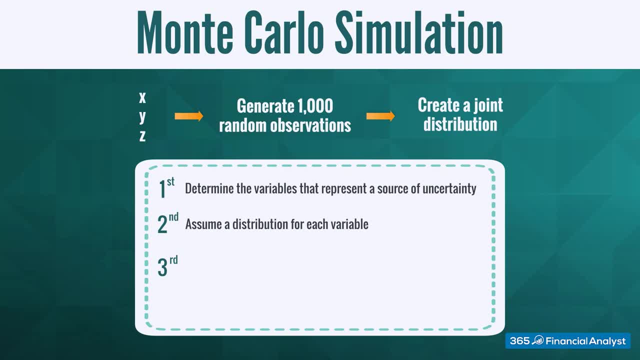 Once we have chosen the different types of distributions describing the random variables, we need to carry out iterations with possible realizations for these variables. And fourth, by repeating the third step, many, many times, hundreds, but more likely thousands of times, we would be able to observe. 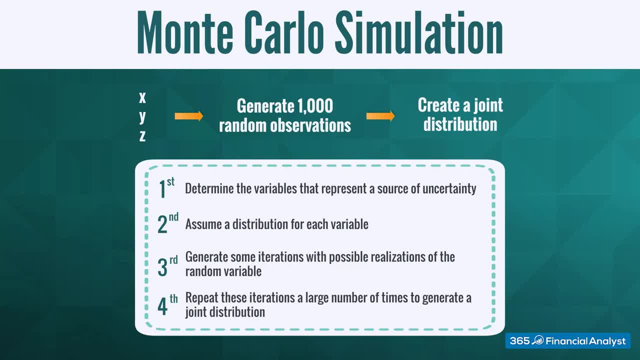 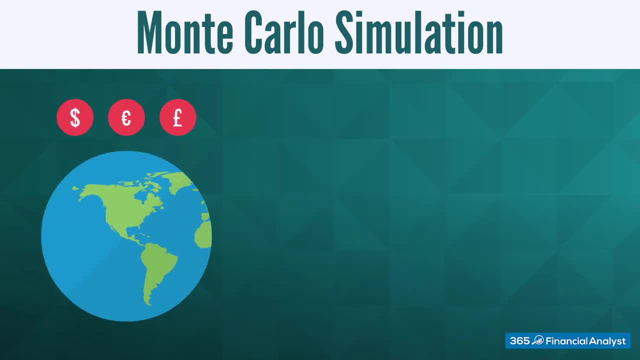 a large number of possible realizations paths that ultimately indicate what could be expected in terms of the mean of the distribution In practice. Monte Carlo simulations find a large number of applications in the world of finance. Some examples are options and other derivatives pricing models. 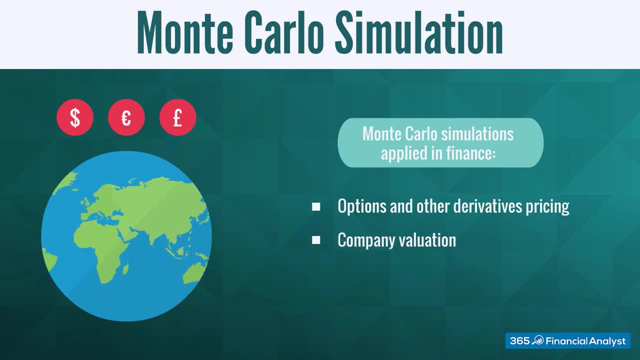 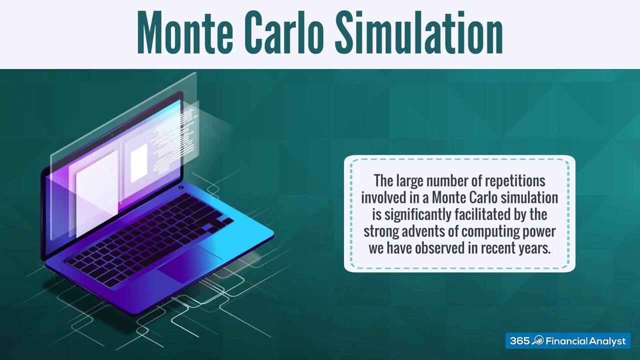 when complex features are involved. Company Valuation To cross-check results obtained through a DCF. use Monte Carlo to triangulate And risk management. Monte Carlo is frequently used for a value-at-risk estimation And volatility modeling. The large number of repetitions involved in a Monte Carlo simulation. 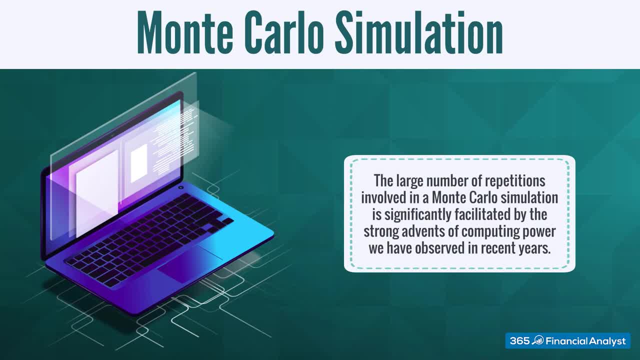 is significantly facilitated by the strong advance of computing power. we have observed in recent years, Running a Monte-Carlo simulation with a very large number of observations does not represent a significant difference between awesome and bad Thank you issue for most models nowadays. this technique is very useful whenever an 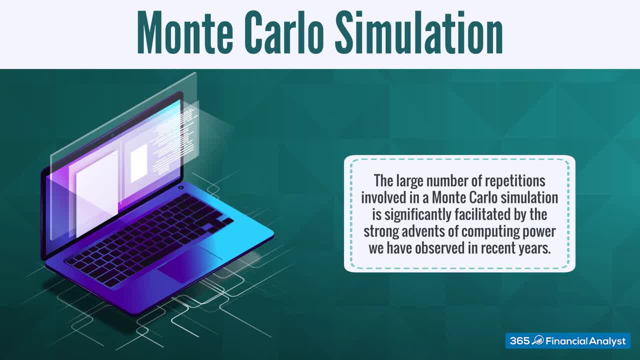 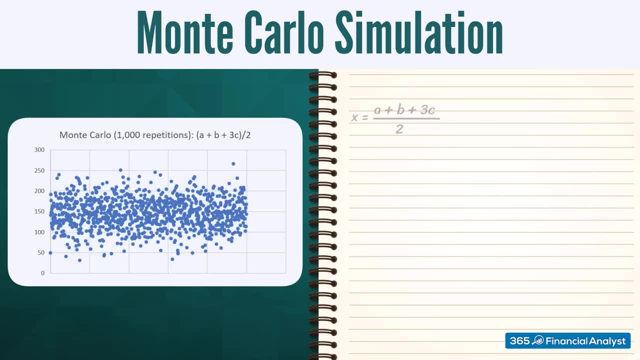 analyst would like to gain an idea of the different possible realizations that could be obtained through a given distribution function. for example, if a distribution function considers three possible variables influencing an assets price, then by testing for different values of these variables, we could obtain a good idea about the possible prices of the asset, provided that the